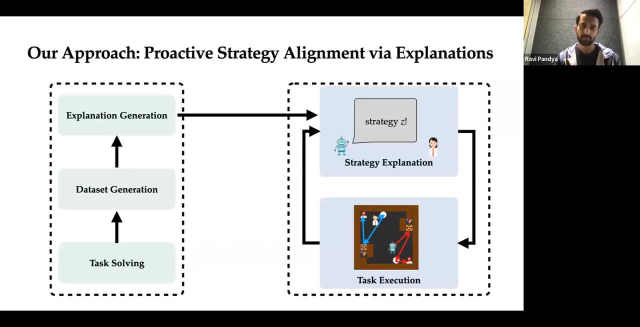 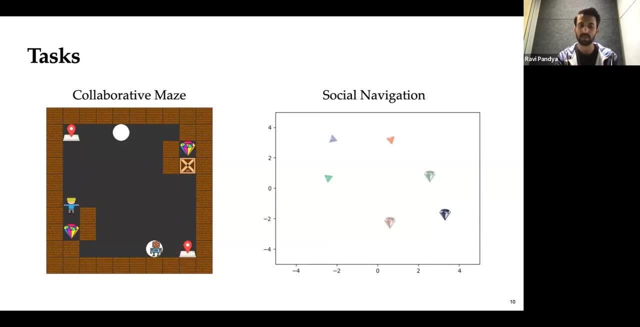 an explanation from the robot and then executes it. And we focus on these two tasks. First, on the left, is this collaborative maze task where the two agents are trying to get these jewels and bring them to the goals. The problem is that they're blocked by doors, so one agent has to step on a button to unlock the door, while the other 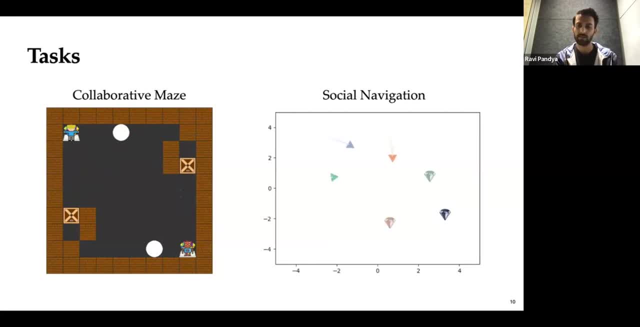 agent grabs the jewel And the social navigation task. the three agents are trying to grab their own jewels without colliding with each other, and you can see an autonomous rollout of three agents successfully coordinating and completing this task without colliding. So, before jumping into 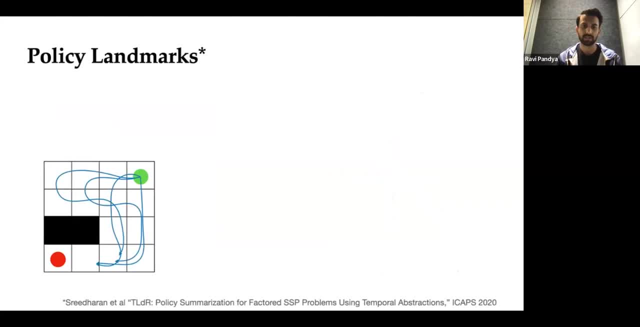 our approach. we have to talk about what we're going to talk about today. We're going to talk about policy landmarks. So let's say we have this data set of all these trajectories from the start to the goal. The set of policy landmark states will be all those states that pass through every 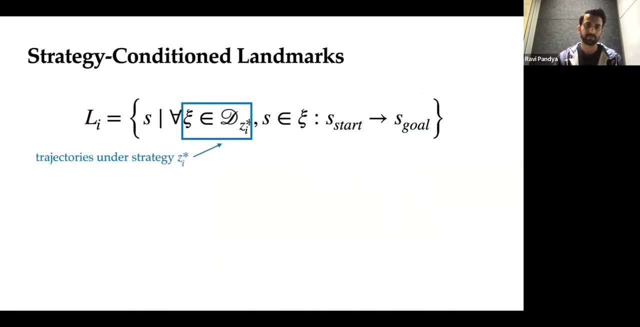 single trajectory. So that's these orange states on the bottom. And we extend this idea by introducing strategy condition landmark states, which specifically look at all of these states that are in just the trajectories under a particular strategy zi. So in our social navigation example, here's all the trajectories from the start state to the goal state for one. 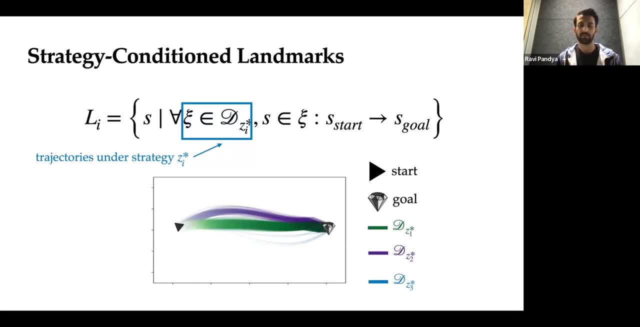 of the agents and we can partition this into three different data sets. So in our social navigation example, here's all the trajectories under a particular strategy, zi. So we can partition this into three different data sets and find the strategy condition landmark states for each of these data sets. The trouble is that this might be not separable in xy space. 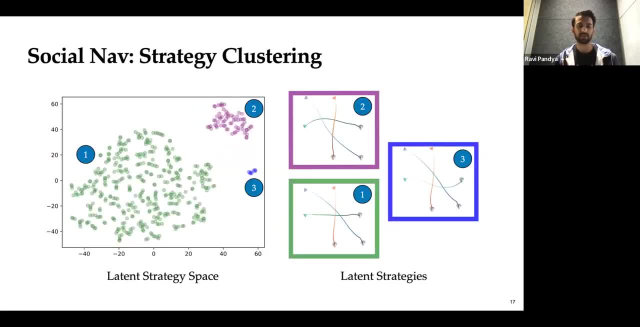 So instead we think about doing this clustering in a latent strategy space, and you can see that if we do uncover some latent strategies, then this space might be very easily separable into these three big clusters, like it is in this task, where each strategy corresponds to which agent goes. 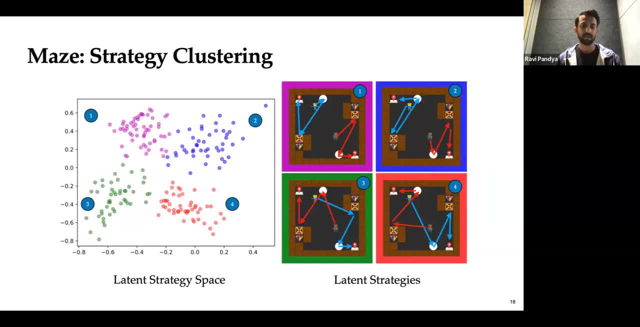 first in picking their goal. And in our maze example, we can use imitation learning to uncover some latent strategy space that's learned through an encoder, decoder structure where we can directly cluster this latent strategy space and find that each strategy corresponds to a different ordering of which agent goes to which goal first. So here's one example: strategy that's generated. 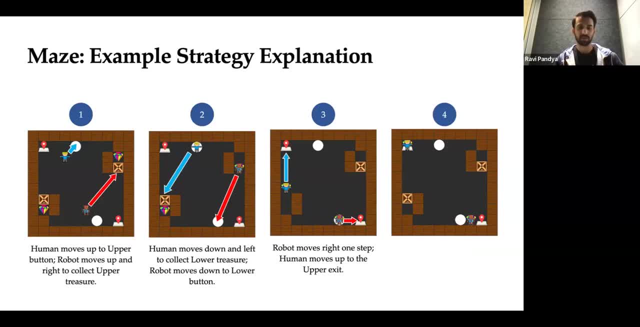 from our task, from our explanation generation pipeline for this maze, and then the robot gets the jewel and the robot goes to the bottom button and the human gets the jewel before leaving the game, and these text on the bottom is actually generated by a large language model. So in our social navigation task, here's one example strategy for 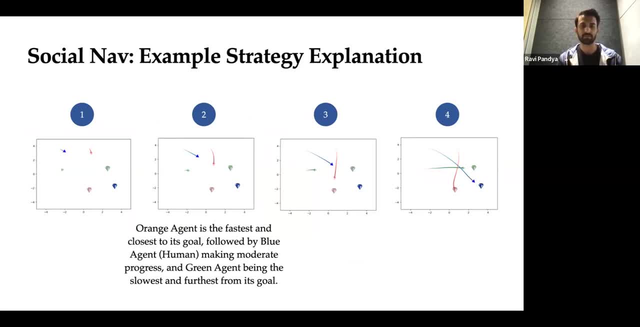 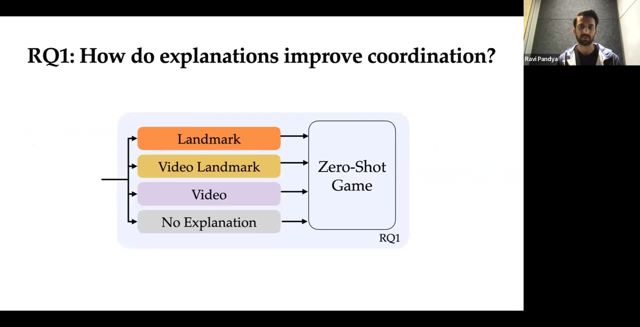 this task where the first, the red agent, goes to their goal, then the blue agent goes to the goal and finally the green agent goes to their goal. So we ran a user study and we had a bunch of different research questions. First we were curious how explanations improve coordination. 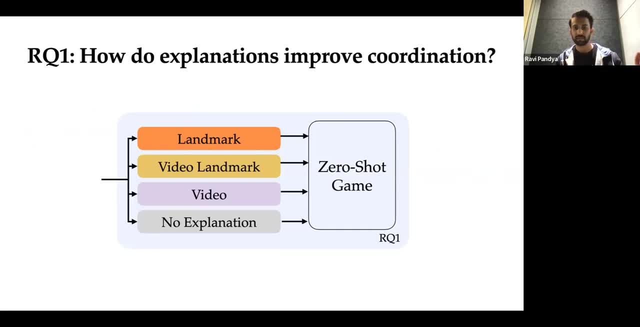 between the human and the robot. So we have different types of explanations that we're testing: Landmark and video. landmark are our strategy condition, landmark for each explanation, generation methods, and then video just shows the trajectory that corresponds to the strategy cluster for each, the strategy cluster center for each strategy and no explanation. 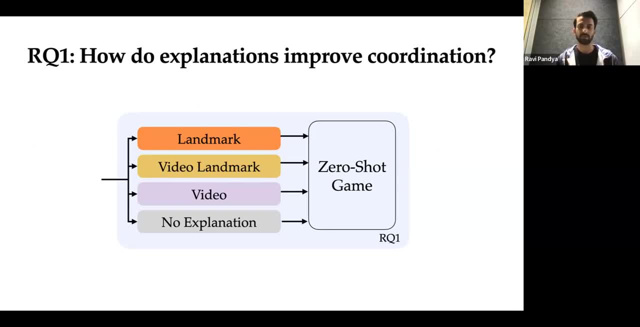 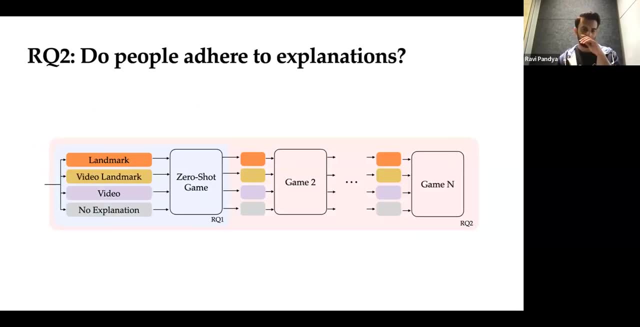 just means that the person gets the rules of the game but does not get a particular explanation of a strategy. So for our second research question, we were wondering whether people adhere to different explanations over time. So we show the person explanations and then play different games. 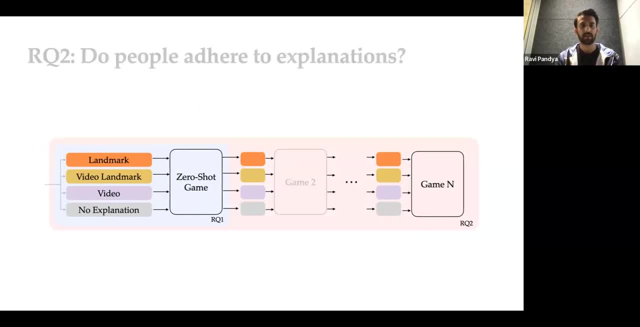 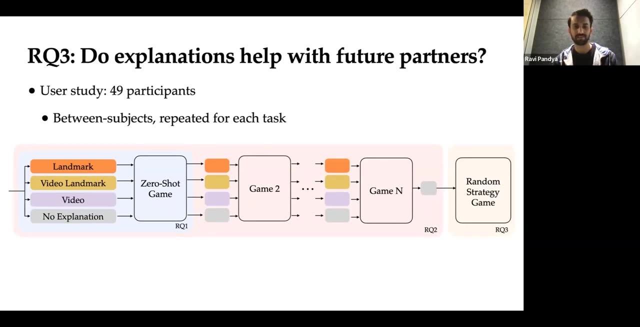 for the number of different strategies there are in each task. Finally, people are shown no explanation and then play a random play, a game with an agent that picks a random strategy to test whether this explanation does help with future partners. and we run a user study with 49 participants. that's between subjects, so each person only sees one. 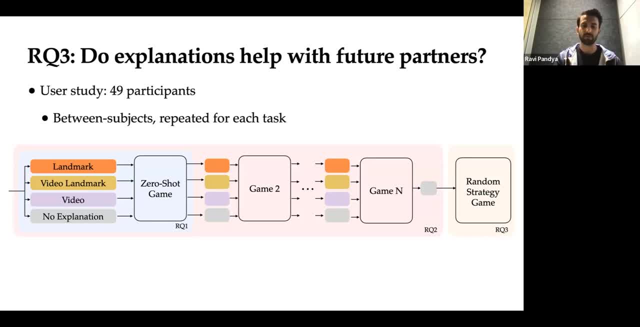 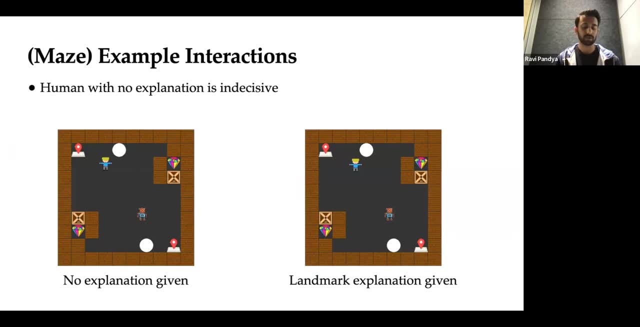 kind of explanation throughout all of their games, and this is repeated for both types of games. So, as an example on the left, you'll see what happens when one user is not given any explanation and they're actually very indecisive On figuring out what they want to do before finally picking this jewel on the top right. 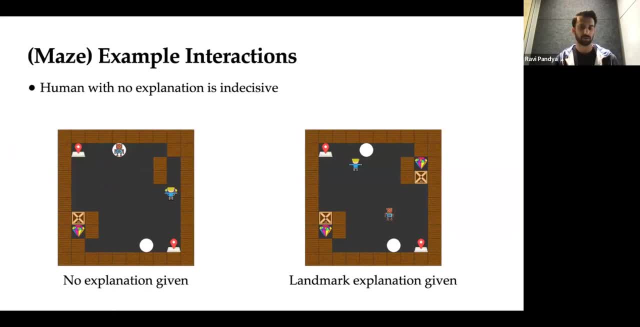 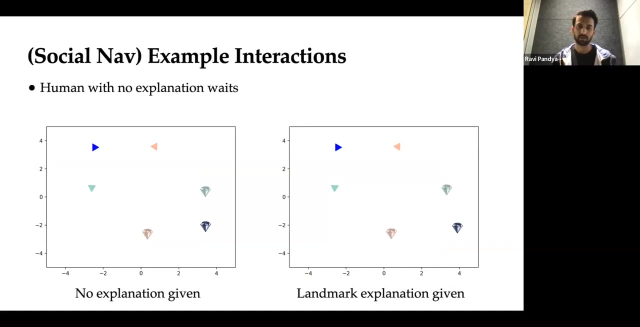 versus if they're given an explanation of this strategy using our method. they're actually very decisive in picking this jewel and it lets them complete this task much faster. So in the social navigation example, the human is in the top left. they're this blue triangle and you can see that. 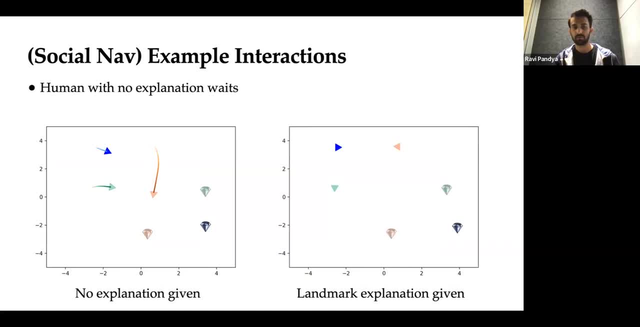 when given no explanation, they're sort of hesitant and they don't understand what to do before they figure out that they should just wait and then cross at the end and get to their goal, versus when they're given an explanation from our method, they understand that actually there was a chance for them to cut in front of this green agent and